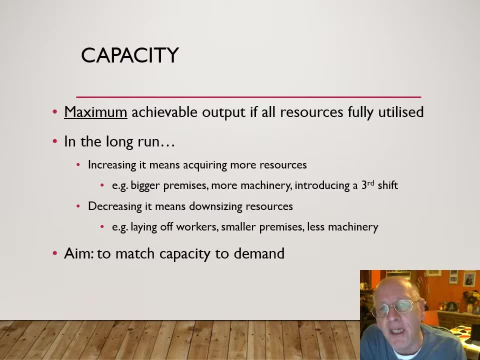 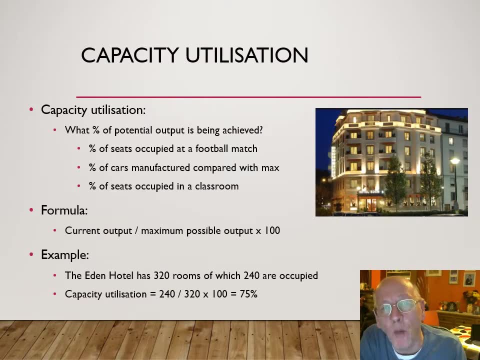 Your broad aim with capacity is to try to make sure that your capacity matches your demand. So if that's capacity, what is capacity utilisation? Well, it's the extent to which your capacity is currently being met. So if, for example, your pint pot is half filled, 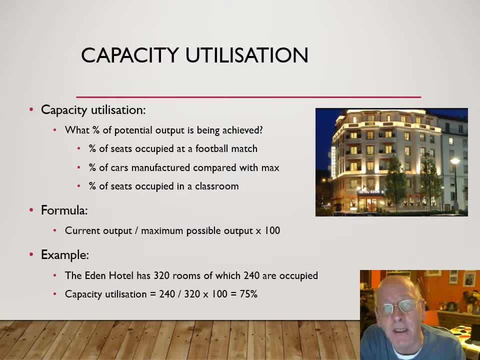 then your capacity utilisation is 50 percent. If you're watching a football match and a third of the seats are unfilled, then you've got a capacity utilisation of about 66, 67 percent. Obviously, big implications during Covid because theatres and football matches aren't allowed to have all of their seats filled. 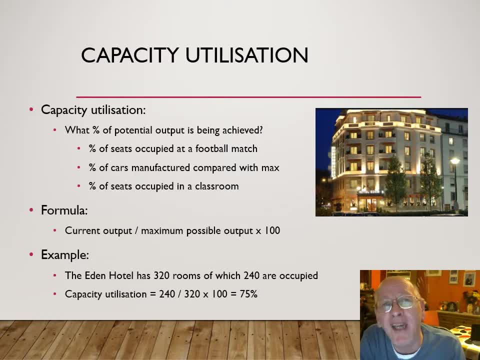 The formula, ever so straightforward, is your current output, what you are producing now, divided by your capacity, multiplied by 100 percent. Example down the bottom there, If you're a hotel, you've got 320 rooms, 240 of them are occupied. 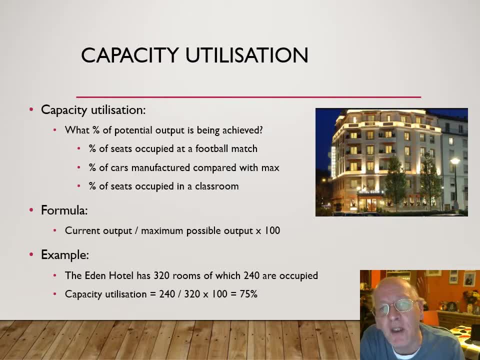 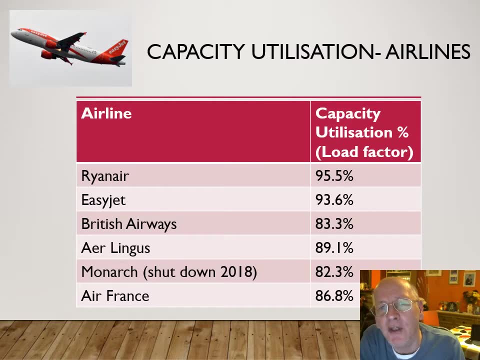 That means a quarter of them aren't, So your capacity utilisation is 75 percent. If we apply this, the term for capacity utilisation they use in the airline industry is the load factor. So in other words, it's the percentage of seats on an aircraft that are actually filled. 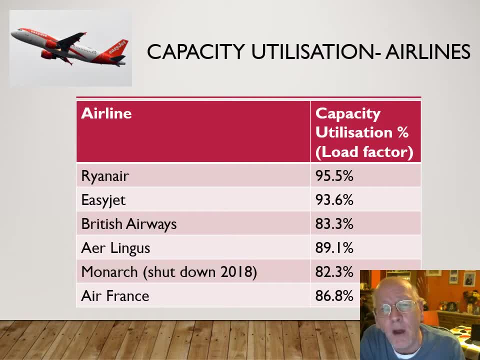 And if you look at some of those figures, they are incredibly high: Ryanair over 95 percent, EasyJet over 93 percent British Airways. about one in six seats is unfilled. Not that much of a problem for British Airways, because they are much more expensive than Ryanair or EasyJet. 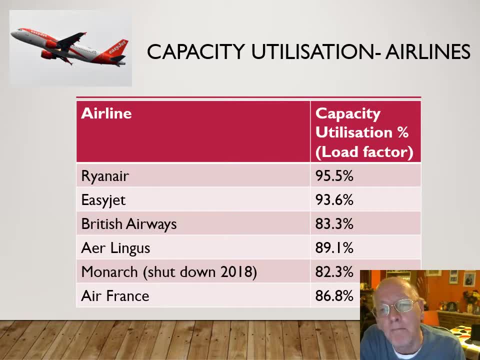 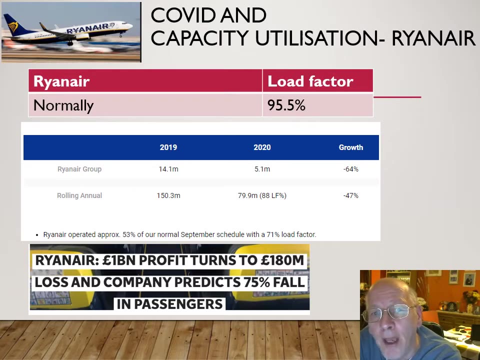 So their profit margins are that much higher. But you will spot Monarch running with 82.3 percent shutdown. Thomas Cook also was relatively low before it shut down If you look at the impact of COVID on capacity utilisation for one leading airline, Ryanair. 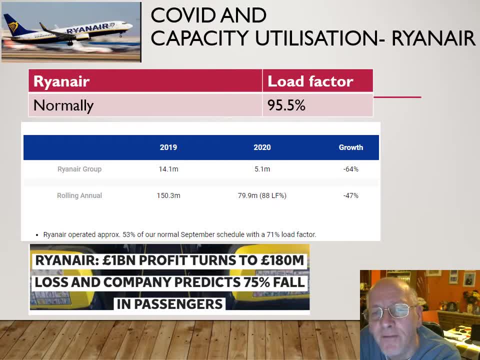 you'll see that normally they have a load factor of 95.5 percent. Well, in 2020, in September, they were running 53 percent of their normal flight. In other words, half of their craft that they would have used last year, they are not using. 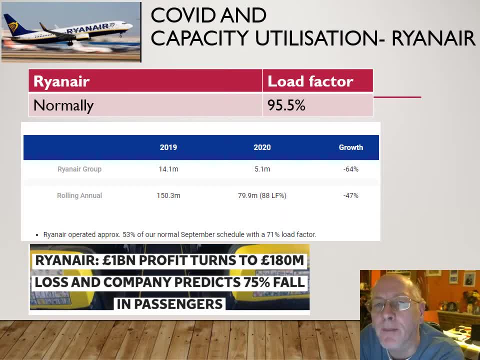 And those that are being used have got a 71 percent load factor, So they're 30 percent empty as opposed to four and a half percent empty. Now the implications of that in terms of their profits. This was taken from a headline on the 2nd of November 2020.. 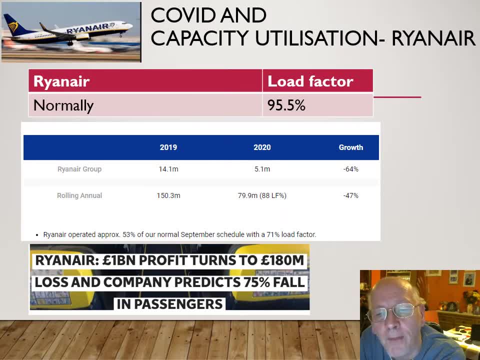 Last year they made a one billion pound profit. This year, as a result of that, they have made 180 million pound loss and they are predicting that moving into the long term. So they're currently looking at ways of downsizing to deal with that. 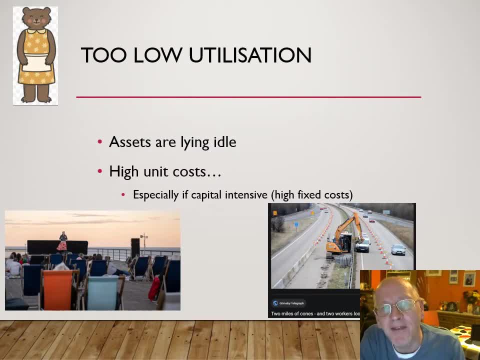 So if we look at the mummy bear scenario, where your utilisation is too low, that means you've got assets that are sitting there doing nothing. It means that your unit costs are going to be high, particularly if you're a capital intensive firm. 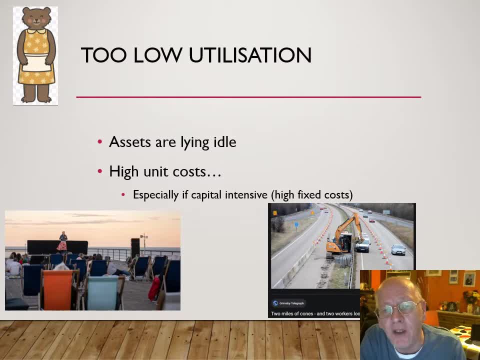 So a couple of examples down the bottom there of underutilisation. On the left hand side you see performance by Eddie Izzard, one of Britain's top comedians, during COVID, where he's performing on the top of a theatre, on the roof of a theatre. 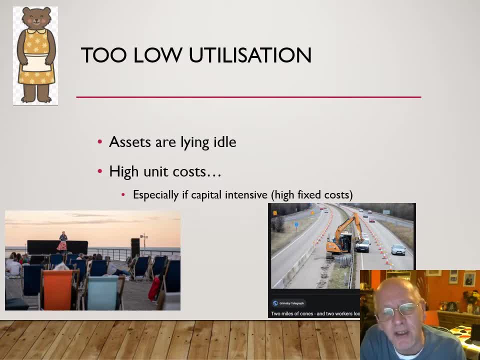 You can see, the social distancing means that there's lots of space that is not being used. On the right hand side you've got a common complaint where drivers drive past miles and miles and miles of roadworks, except they can't actually see anybody working on those roads. 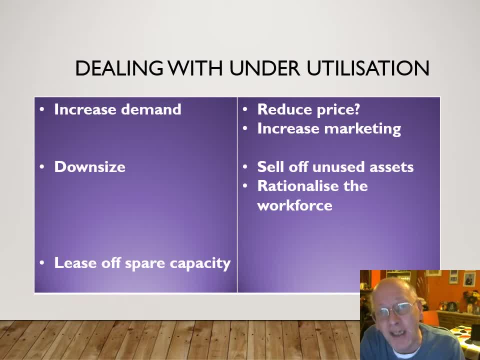 So how can a firm deal with a situation of underutilisation? Well, one thing they could try to do is to increase demand, So the demand rises to capacity. Obvious ways of doing that: reducing your price or increasing your marketing, Or, alternatively, they can downsize. 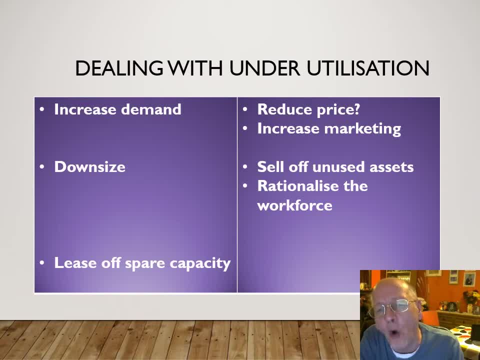 That means selling off your unused assets or rationalising the workforce. If ever you're employed and you hear that your company is rationalising, that should be where you should be looking for a new job, because it means sacking some workers Or they could try to lease off some of that spare capacity to another firm. 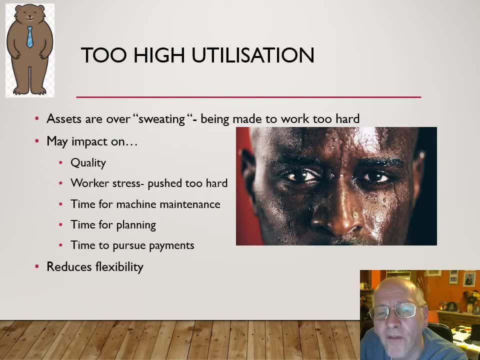 So what about the daddy bear scenario Where you've got too high capacity utilisation? Well, broadly speaking, the higher your capacity utilisation, the lower your scope if there's a change in the market, particularly if there's a further increase in demand. 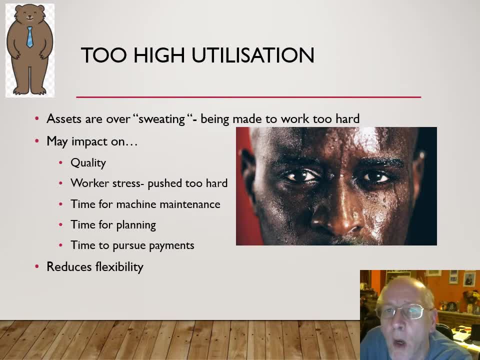 How can you cope with that if you haven't got spare resources? One of the terms that you use with capacity utilisation that's high is the sweating of your assets, And it may be that your assets are sweating too much. You're spending so many of your resources. 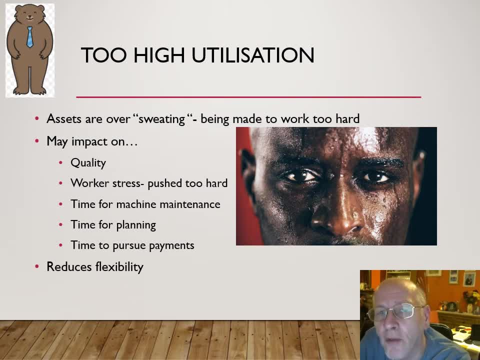 Trying to chase up current demand that you perhaps lose sight of the future. You might find there's quality implications because you're concerned with quantity. You might be over pushing your labour force because people can break down. You might be reducing the time that you're using for machine maintenance. 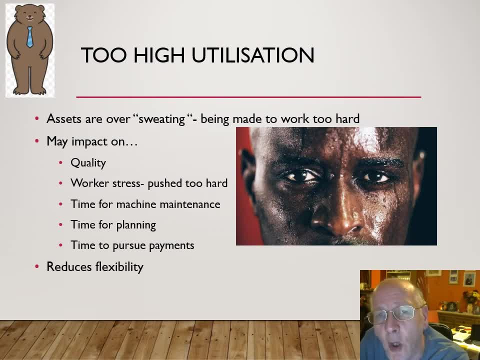 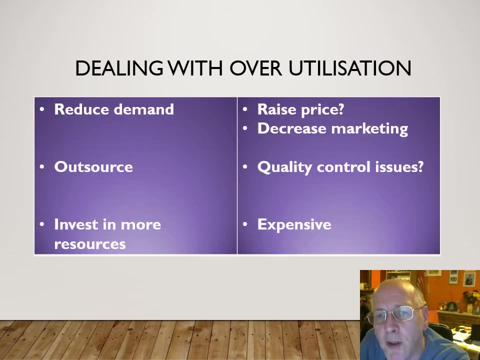 Again, that might have safety implications in the long term, And your management and admin resources might be focused on dealing with the here and now rather than the future. So too high utilisation is not always a good thing. So how do you deal with over utilisation? Well, one thing you can do is you can try to reduce demand so that it's in line with what you can produce, For example, raising price or decreasing your marketing expenditure. You could possibly try to outsource that extra demand to another firm. 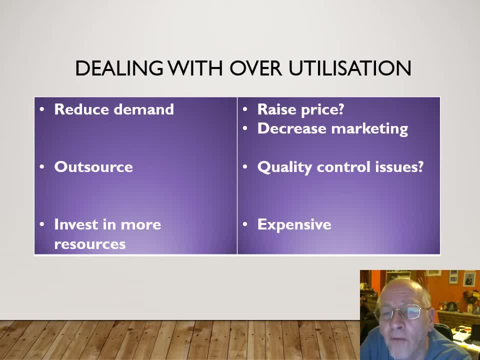 That will obviously bring in implications of quality control, because you are no longer in control, You're no longer producing the goods yourself, Or you could try to increase the scale of your operation. Frequently that's expensive. Think in the football industry about firms that have done that in the last few years. 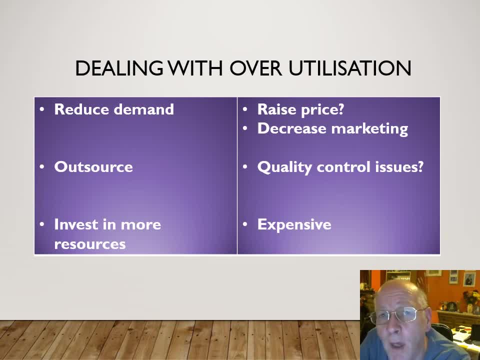 Manchester City, Arsenal, Tottenham, West Ham. Think about the cost implications of that: Very, very expensive to build a new stadium, which is something that often implies- or, at a smaller scale, building a new stand. So what are your? 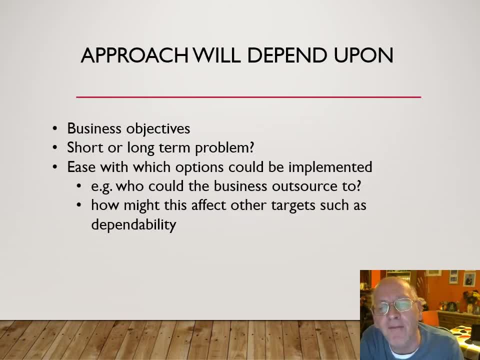 This will depend upon factors that's really useful for moving up the levels. Well, firstly, what are your objectives? What are you trying to achieve? Secondly, of course, do you see it as a short term or a long term problem With COVID? particularly when the government were giving firms help, lots of firms were reluctant to sack their workers because they thought it was going to be over relatively quickly. 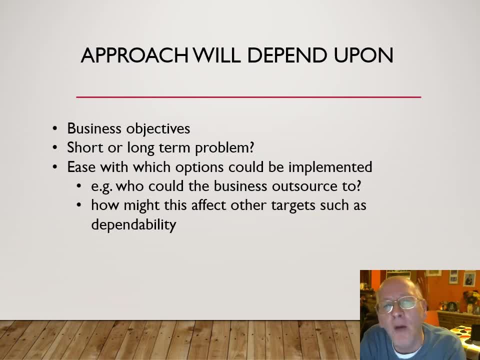 So they didn't want to get rid of that vital resource because they felt they might use those resources again later. And thirdly, of course, how easy is it to do the options that you're faced with? If you're thinking about outsourcing, who might you outsource to?